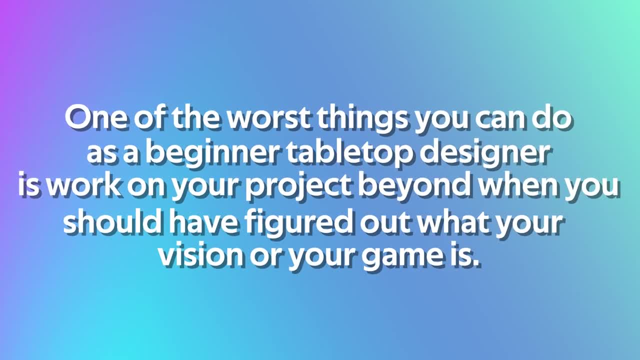 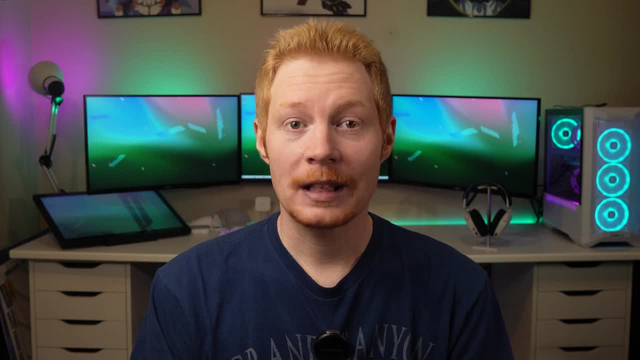 beyond, when you should have figured out what your vision of the game is. Define your game's theme and concept. Try to identify a central theme for your game. What is the story you're setting? What emotions or experiences do you want your players to have? Do you want your game to be fun? Do you? 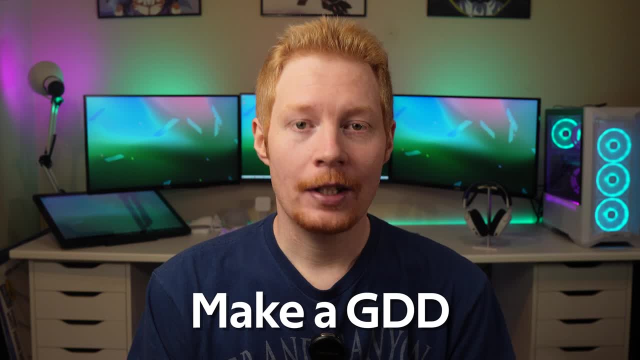 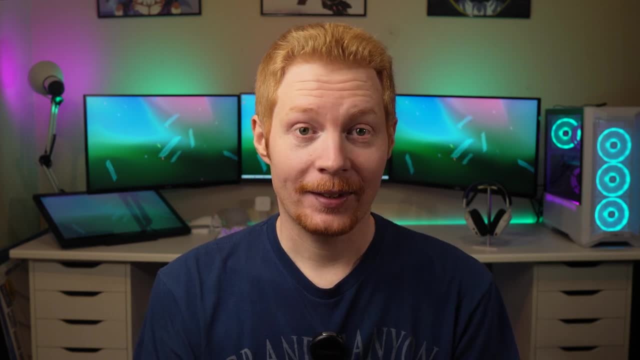 want your players to feel or have. Create a game design document where you write down all your thoughts, ideas and goals for your game. One thing I'm notorious for is getting defensive of a mechanic or system that I've come up with. Sometimes I'm so excited and proud of an idea that 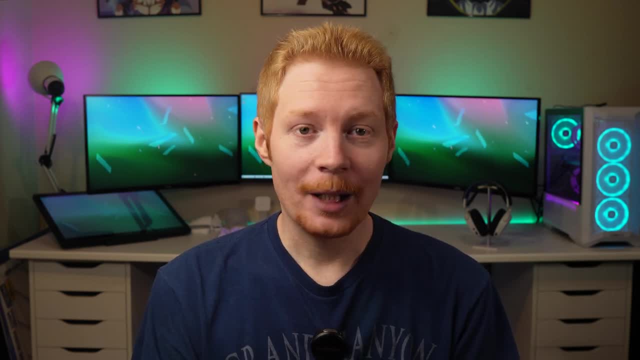 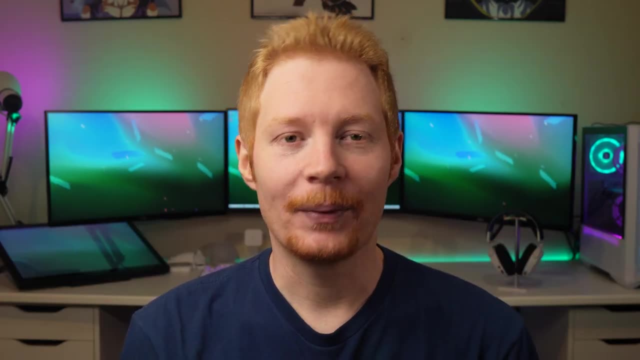 I've had that. I'm quick to defend it Because of course I know what problem it's there to solve and I have a good idea on how it works and how it could be cool. My darn brain can't formulate words in a coherent manner to explain ideas properly, so I end up talking about the idea. 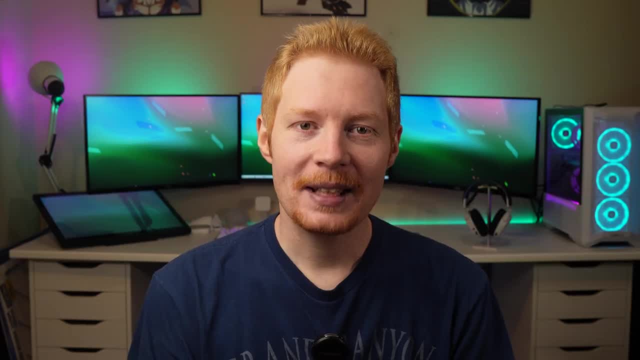 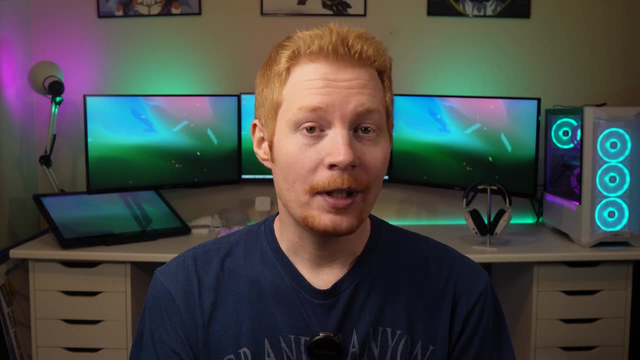 in vague ways and only leave people more confused. This always seems to happen when someone else is trying to tell me that there is an unbalanced mechanic in my game. Again, it's easy to justify or even think of things as lesser evils, but if you take a second to put yourself in your player's shoes, you'll quickly realize that. 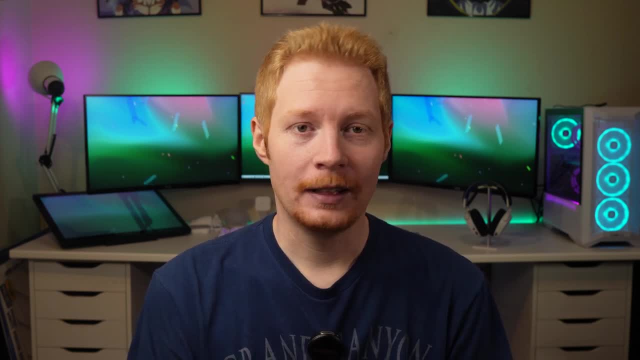 unbalanced mechanics can ruin your fun. Even the impression or feeling of imbalance can ruin the experience. So do what you can to temper that part of yourself. Listen to your players and make sure you reflect on each playtest and pay attention to the pain points that others bring up. 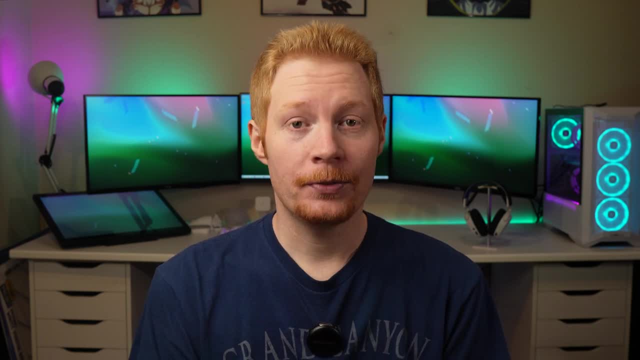 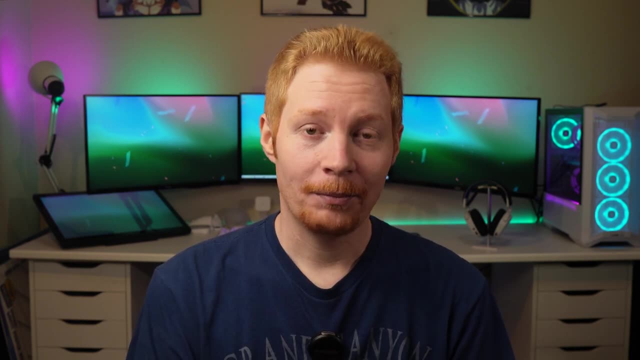 It might feel like whack-a-mole, but remove unbalanced mechanics wherever you find them. The solution to this is linked to the worst mistake you can make as a board game designer, The number one reason your game can fail. More on that soon. 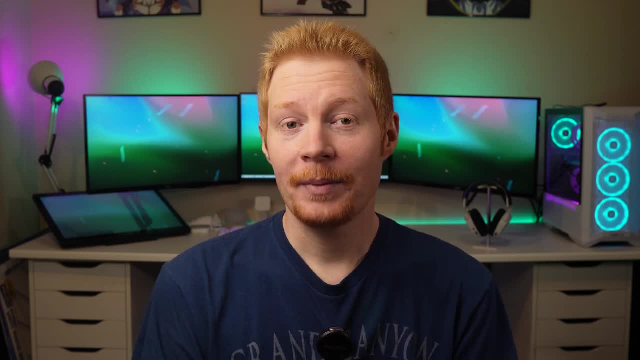 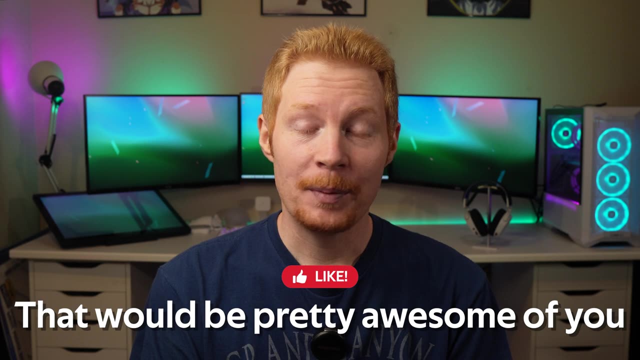 But first I just wanted to stop real quick and say thanks for watching my video. If you would take just a moment to hit that like button, then you would be helping me get one step closer to making my game a reality. That'd be pretty awesome of you. It also helps others. 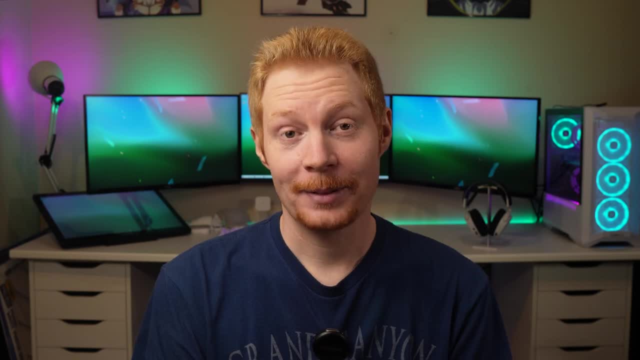 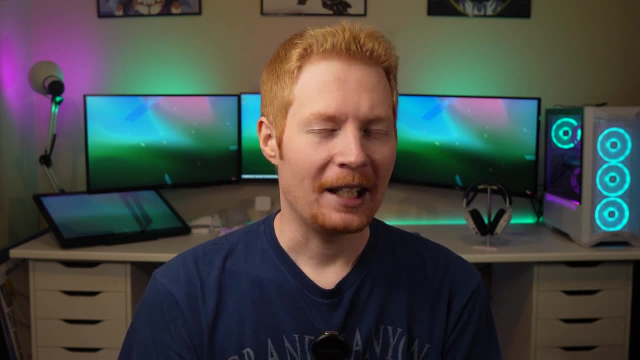 like you, find my content and learn how to avoid falling flat on their face. What is the easiest thing to spot When you're playing a new game and learning all the rules? have you ever gotten the feeling that this might be more of a challenge than you were expecting? But not because the 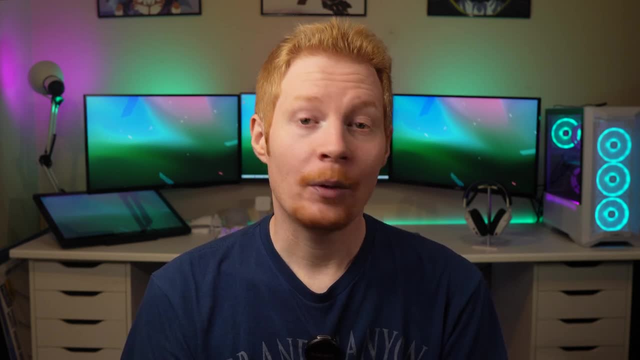 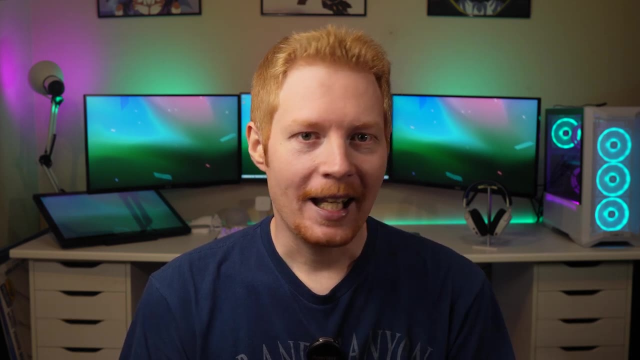 game is hard. As you're playing, have you ever felt like things are needlessly convoluted and the way you expected things to play out isn't the obvious solution that you thought it'd be? Is it as easy for you to spot as it is for me? Have you ever played a game where you need to? 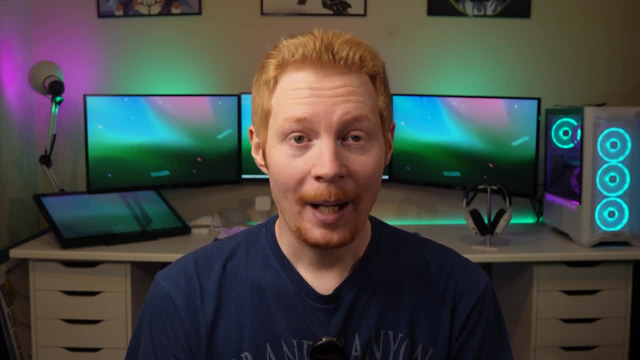 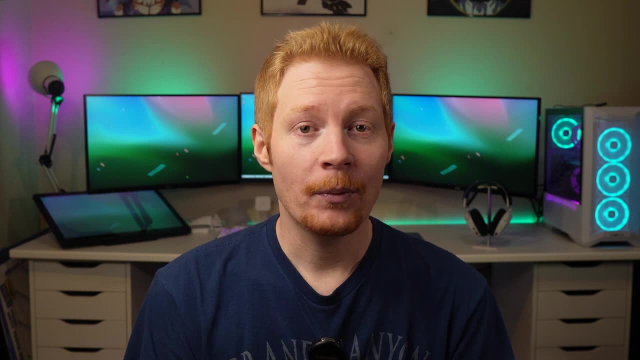 leave the rulebook open on the glossary or reference page just to play that game. When I'm playing games, the easiest thing to spot is overcomplicated rules. When you're designing your game, simplify wherever you can. Find ways to remove redundant mechanics. 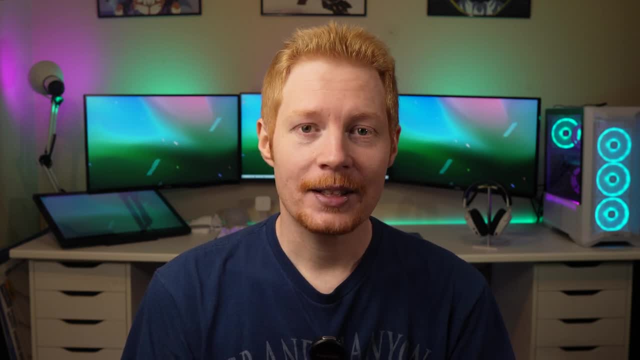 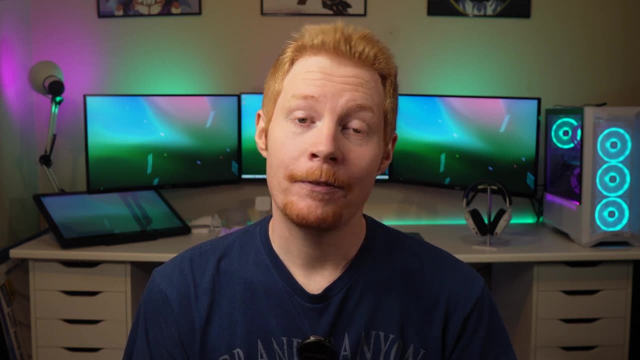 and excessive rule. exceptions or special cases- I'm not sure if this is the right term, but it seems to fit. Aim for elegance. It's the concept of two birds with one stone. Try to find solutions that fix multiple problems. Elegant solutions. 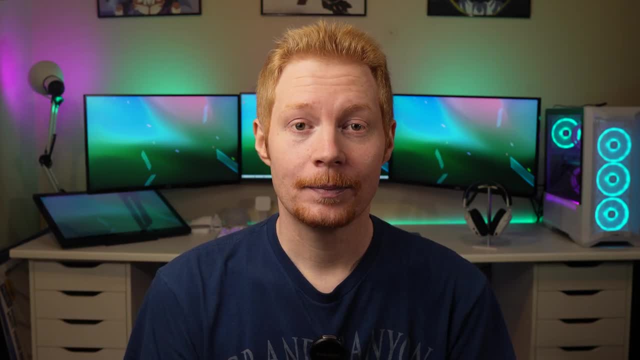 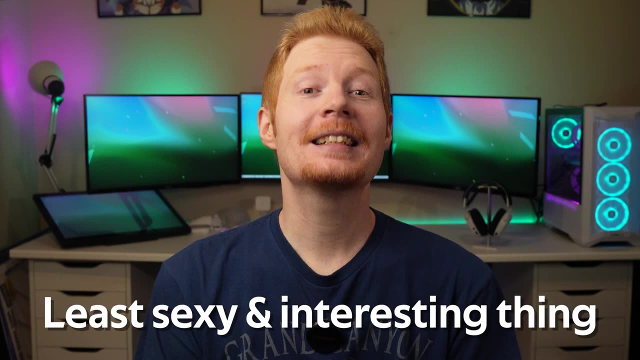 By doing this, your game will eventually be a tight and focused experience. We're getting closer to the number one worst mistake you can make. Have you figured it out yet? But before that, we need to talk about the least sexy or interesting thing about making a game. 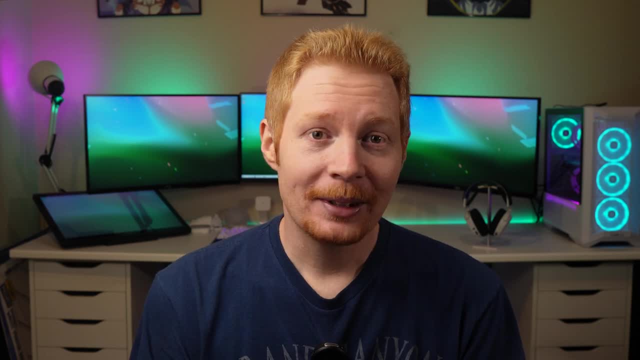 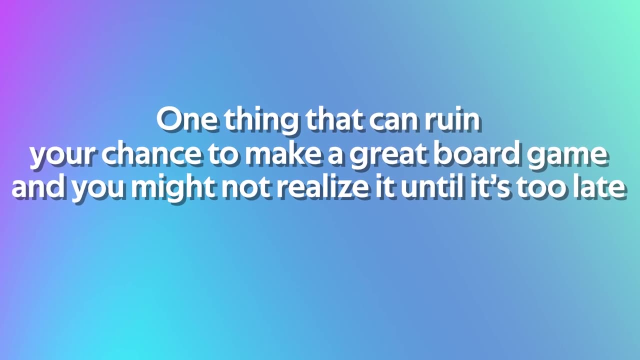 At least it is to me. Maybe this is your favorite part. This is similar to the first point about vision, but more specific. This is one thing that can ruin your chance at making a great board game, and you might not realize it until it's too late, And it involves everyone's favorite Market. 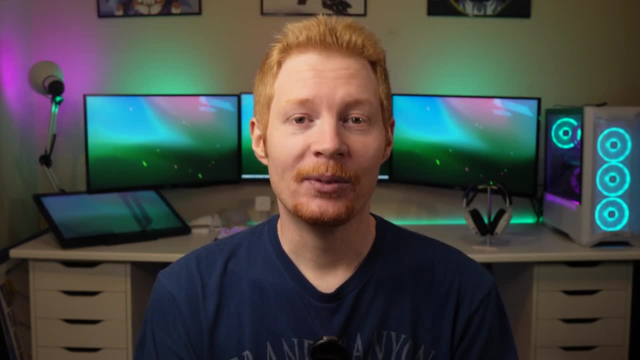 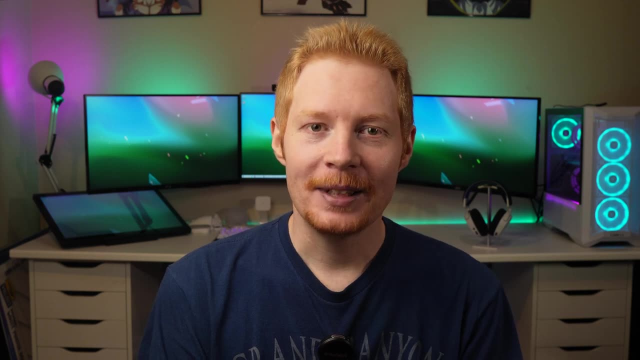 research. I don't know why, but this seems to be the one thing I tend to avoid. Have you ever played a game and thought, yeah, that was fine, I guess I'd play it again, Only to never find a reason to pull it back off the shelf? Games like those collect dust- not because they're bad, In fact. most of them are very well designed and a treasure trove of great ideas to study. The real problem is that they're nothing special, Nothing was memorable or interesting about them. When I think about all of my favorite games, they're my favorite because of unique components. 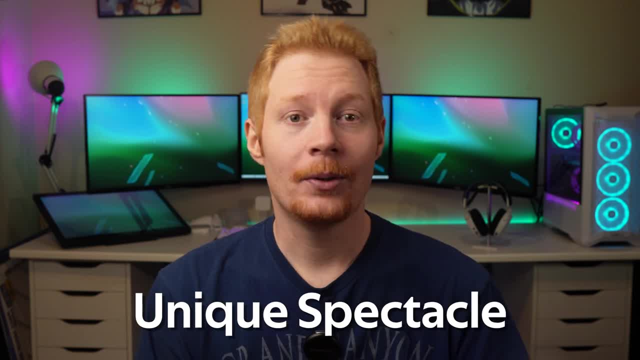 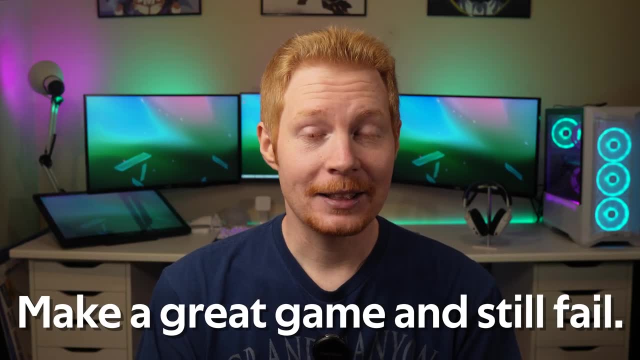 or mechanics I've never seen before, or they have an element of spectacle that makes them great to show off to others. Be sure to consider market viability and differentiation. Without it, you can make a great game and still fail. And on to the biggest mistake you can make. 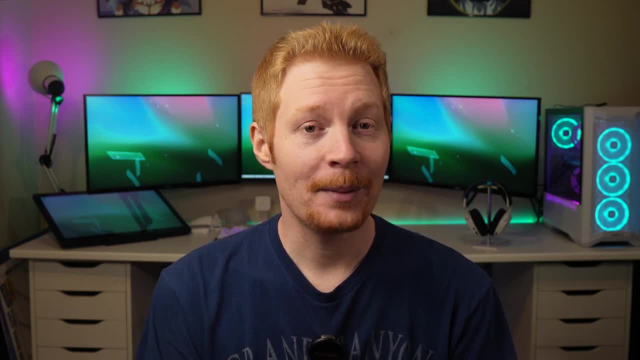 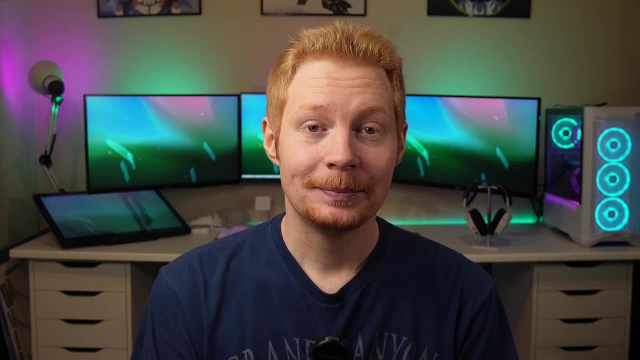 as a board game designer, This is your last chance to guess what it is. Feel free to pause the video and type your guess in the comments- No cheating. It might also be a good chance to hit that subscribe button while you're at it. The reason this is the absolute worst thing you. 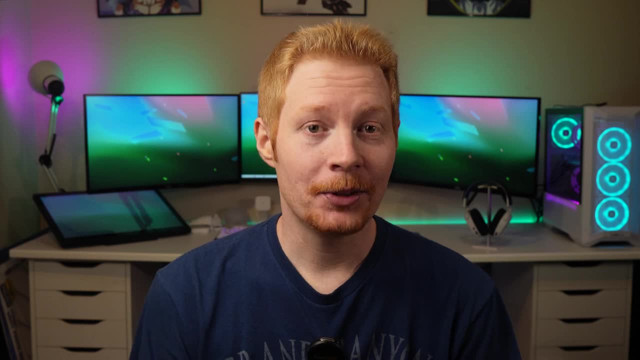 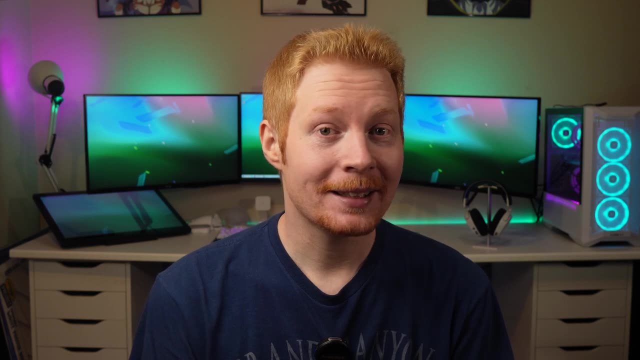 can do as a board game designer is because it will solve all of the other issues I've touched upon already in this video. Do you know how to make a great board game? Surely, it's as simple as following all the steps, checking all the boxes, having great art and a good marketing. 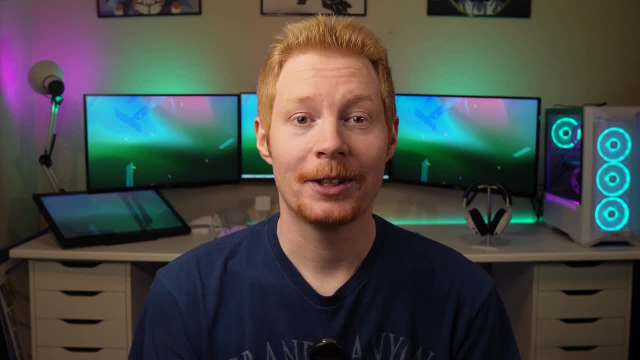 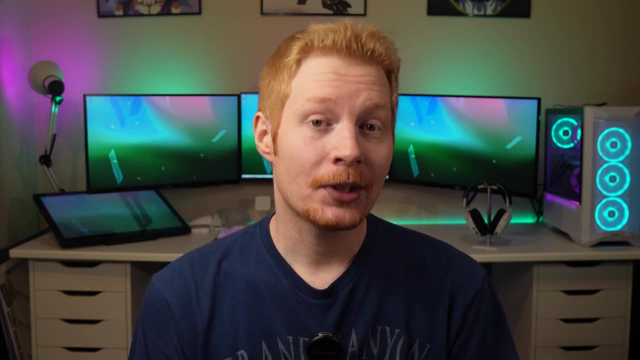 push right, But that wouldn't actually solve all the problems I've touched upon so far. So what can you do to actually make a great game? I harp on this quite often, so maybe it's no surprise, but you solve almost all of your problems through playtesting. 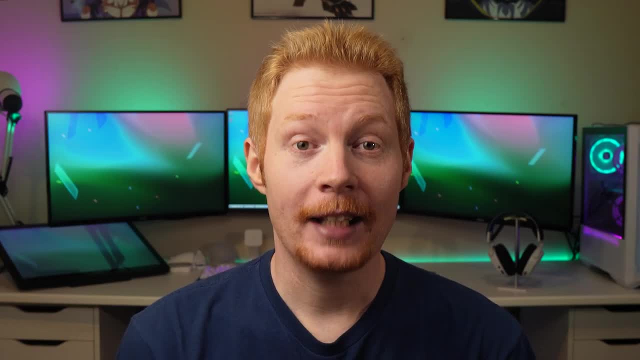 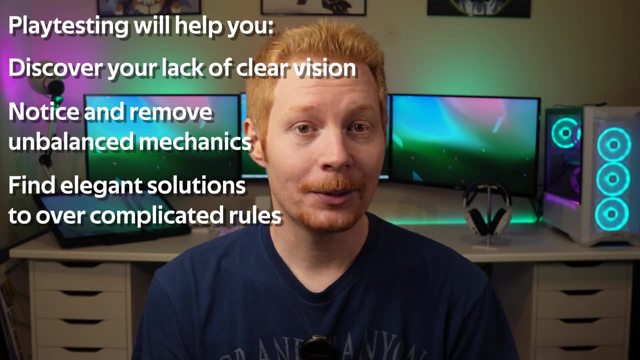 So the number one cardinal sin of a board game designer is not playtesting your game enough. It will help you discover your lack of clear vision, notice and stamp out the unbalanced mechanics, find more elegant solutions to overcomplicated rules and learn if your game